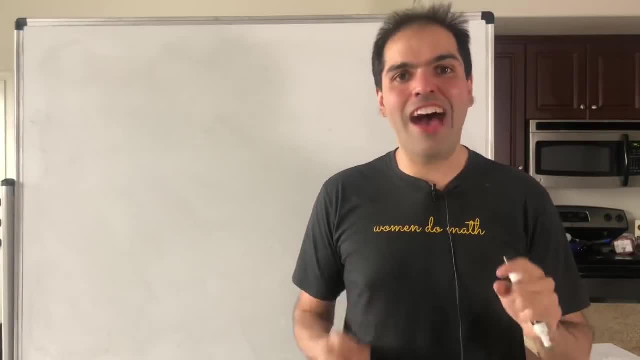 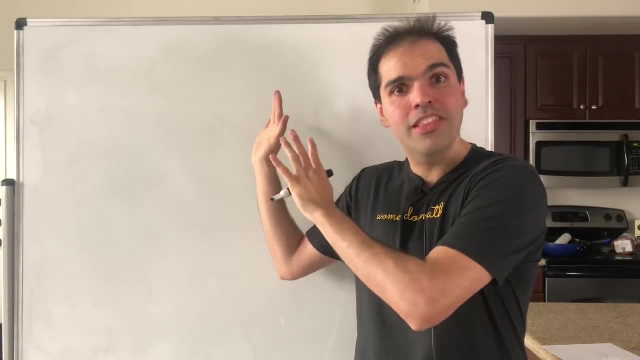 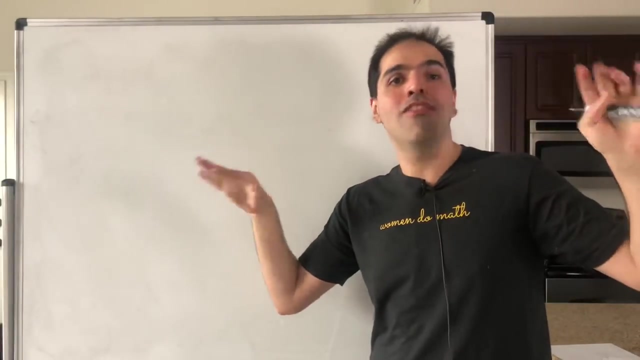 Alright, thanks for watching, and today I want to talk to you about a fact that is guaranteed to surprise you, And you have to understand. if I'm excited about number theory, it means it's a pretty cool fact. Okay, so let's start with something that you probably thought of at some point in your 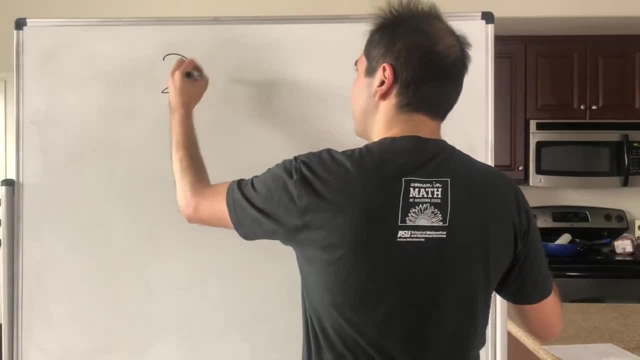 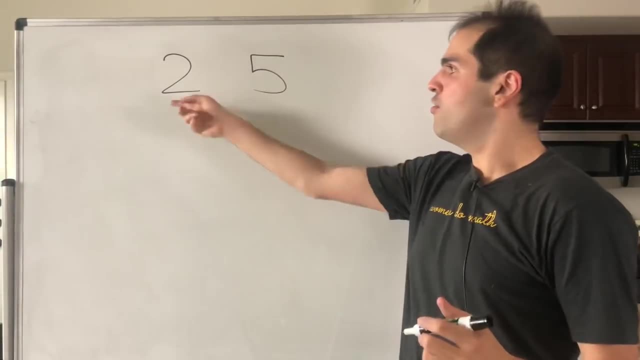 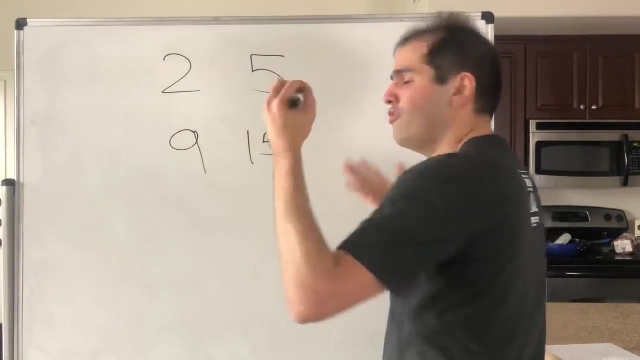 lives. Namely, if we pick two numbers at random, let's say two and five, what are the chances that they have no factors in common? For instance, here two and five have no factors in common, but let's say nine and fifteen, they have a factor of three in common. And let's see how we can approach this. 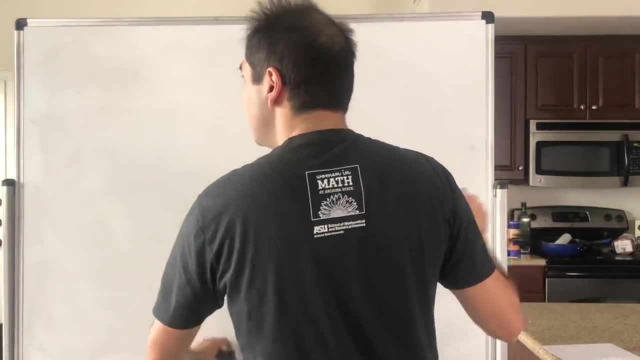 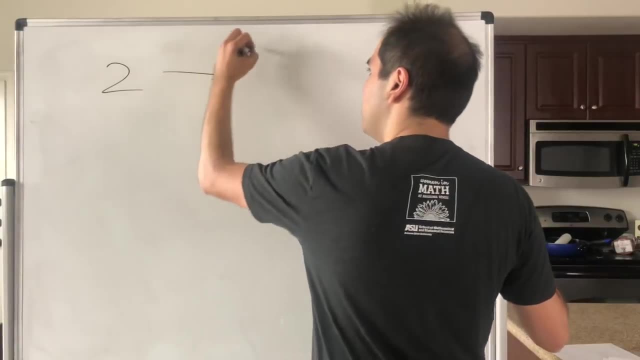 Well, first of all, what are the chances that the number is even? So, what are the chances that the number is divisible by two? Well, one half, because one half of numbers are even. I know Blackpen, Redpen doesn't agree. 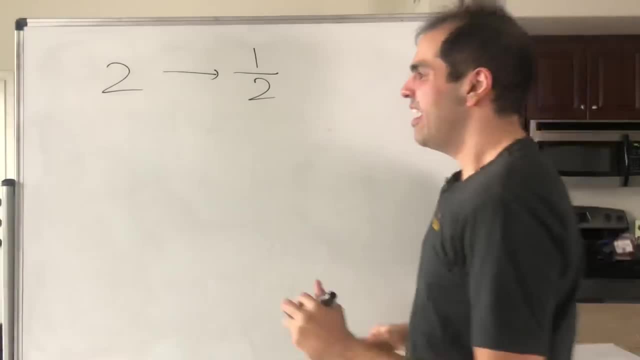 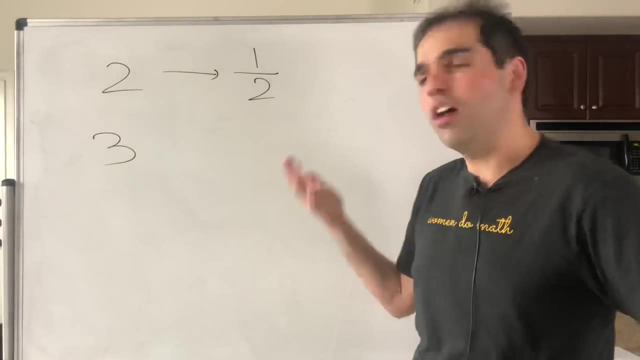 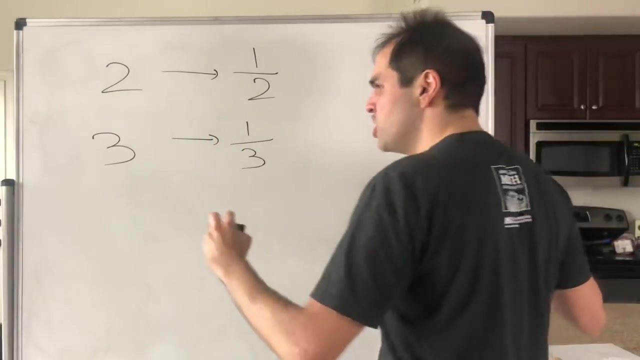 with it, but I think probabilistically this is true. And similarly, what are the chances that a number is divisible by three? Well, one out of three numbers is a multiple of three, So one third. And more generally, what are the chances that a number is divisible by a prime number, p? Well, it's one over p. 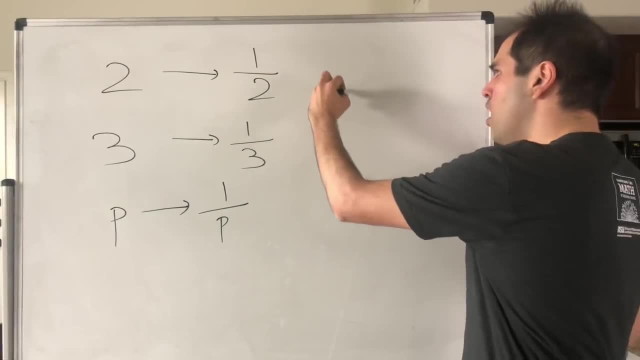 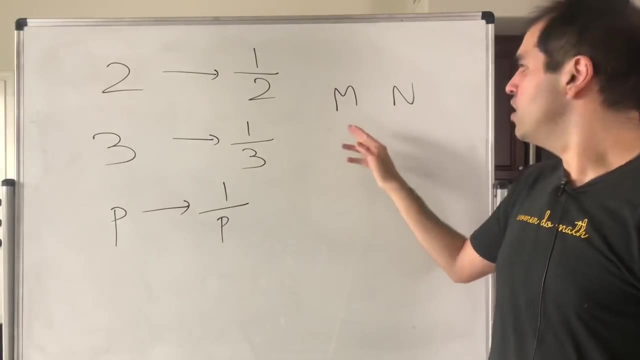 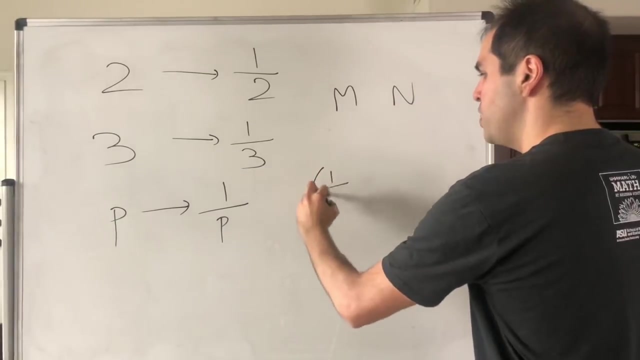 And now look, if we now pick two positive integers at random, well, it is a pretty independent choice. So the chances that both of them have a factor of p in common is just one over p. so for the first, number times one over p for the second: 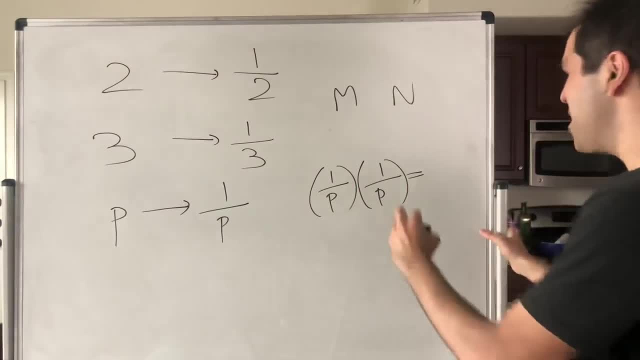 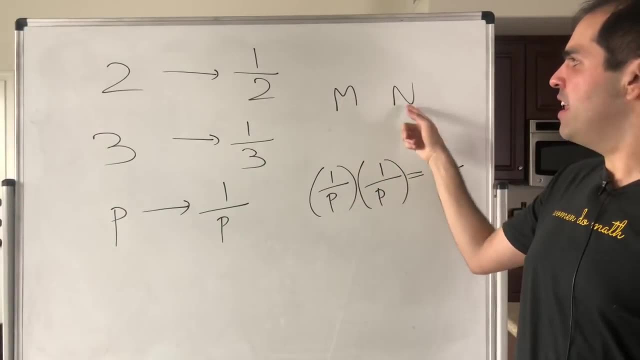 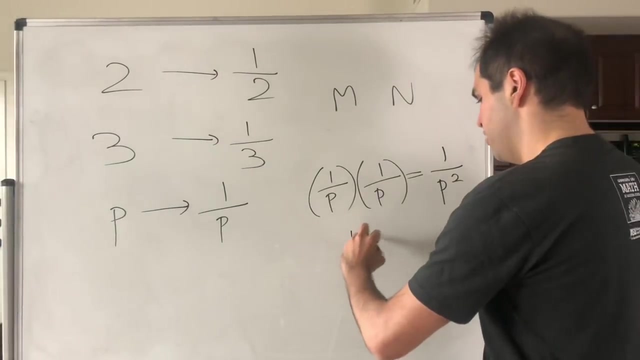 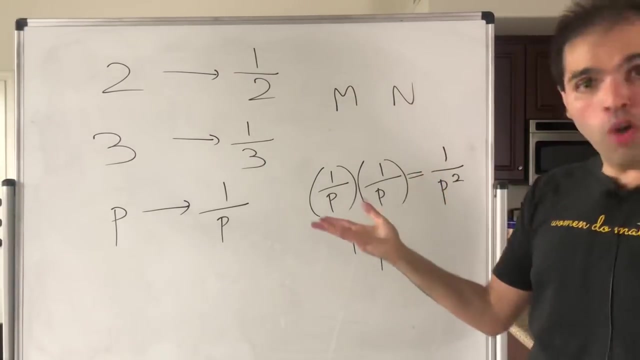 number which, no, it's not one over pi m, but it's one over p squared. In particular, the chances of m and n not having a factor of p in common is one minus p squared. So now the question is: what are the chances that m and n have no factors in common? What does it mean? 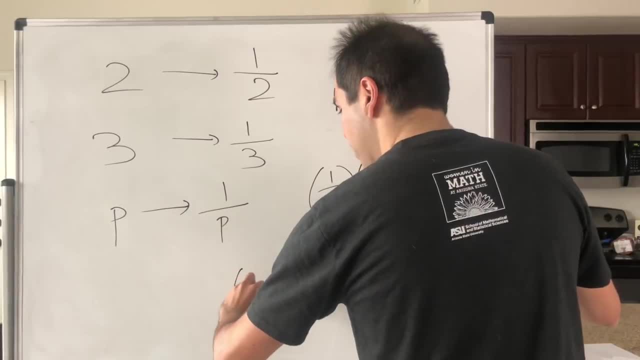 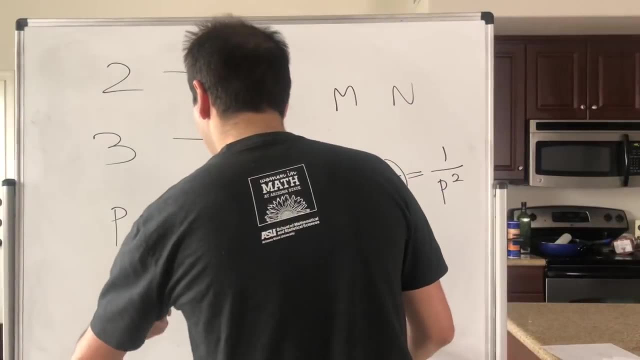 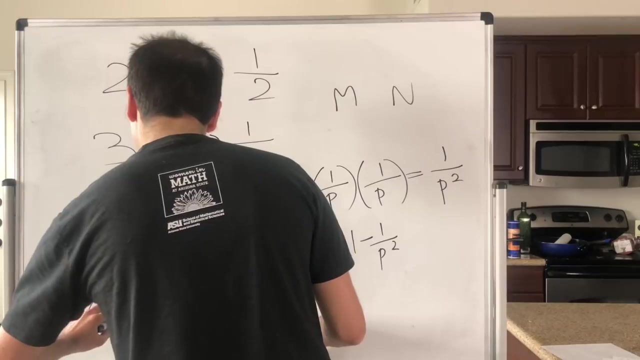 It means they don't have two in common, so one minus one over two squared. They don't have three in common, so times one minus one over three squared, They don't have five in common: 1 minus 1 over 5 squared, etc. etc. 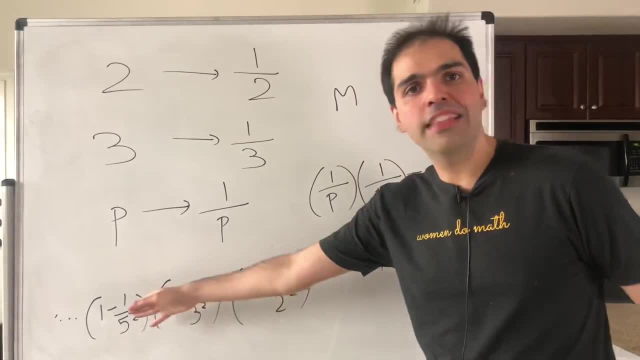 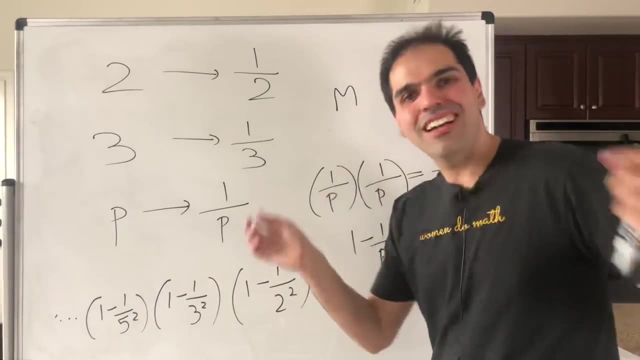 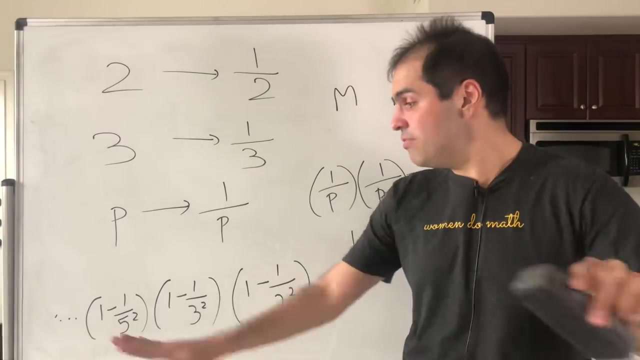 So this is the probability that they have no factors in common, And, of course, now the goal is to write this in closed form, kind of have an explicit formula for this And for this. let's try to cover a problem that seems to have nothing to do with this. 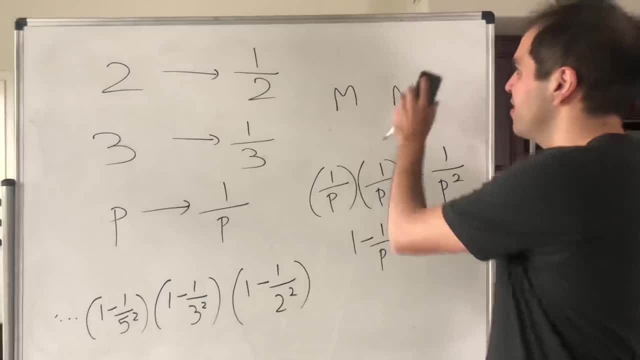 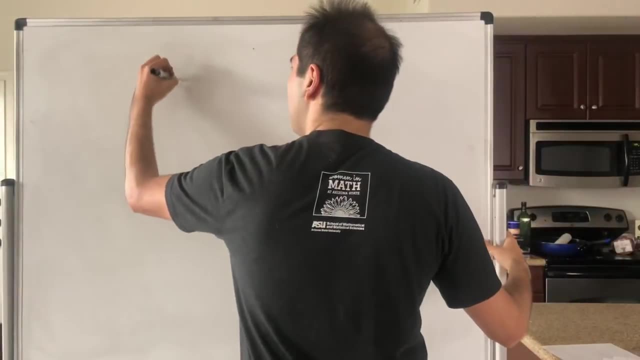 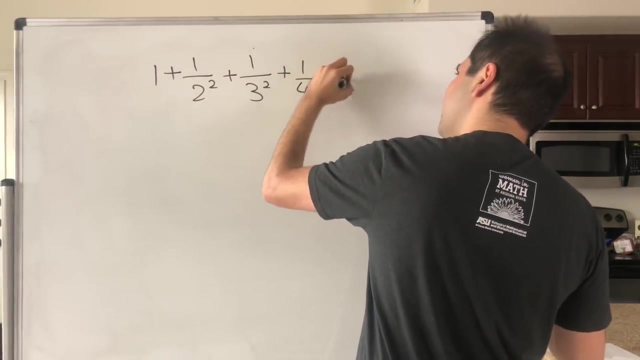 And surprisingly, we'll see that they're related. So part 2, consider the following weird sum: 1 plus 1 over 2 squared, plus 1 over 3 squared, plus 1 over 4 squared, etc. etc. And I have done a separate video on this. 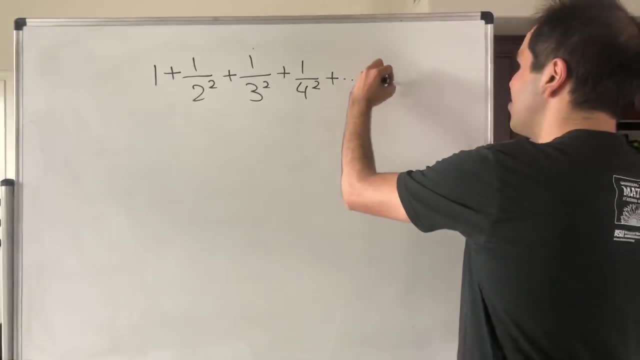 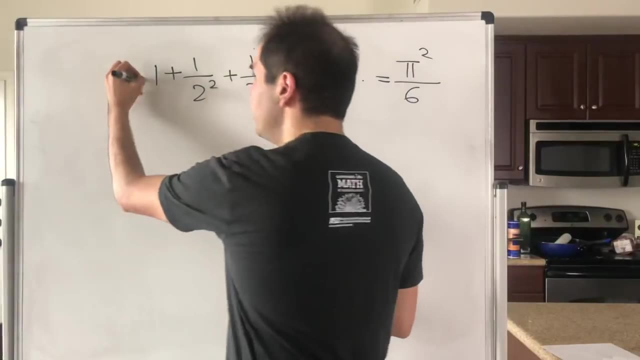 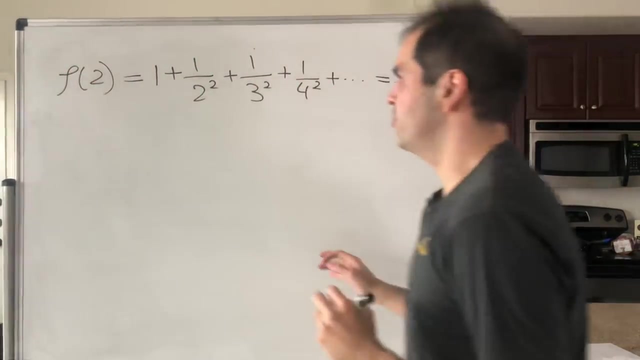 and it turns out this sum is pi squared over 6.. So, using what's called Pachseval's sum- And this, by the way, if you're curious, that's what's called zeta of 2, so the sum of reciprocals of squares. 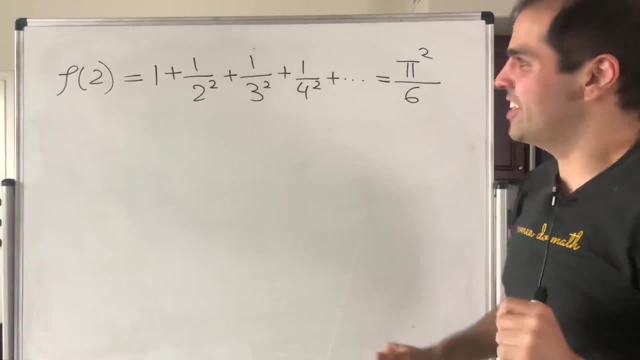 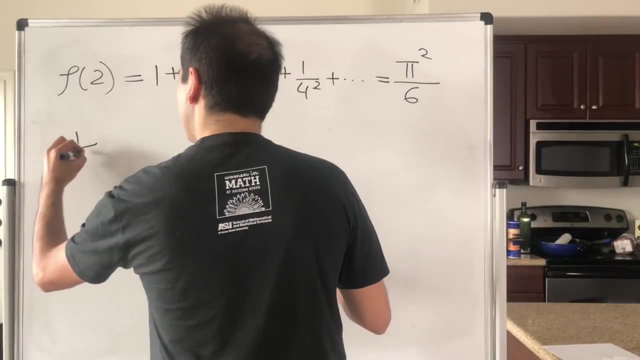 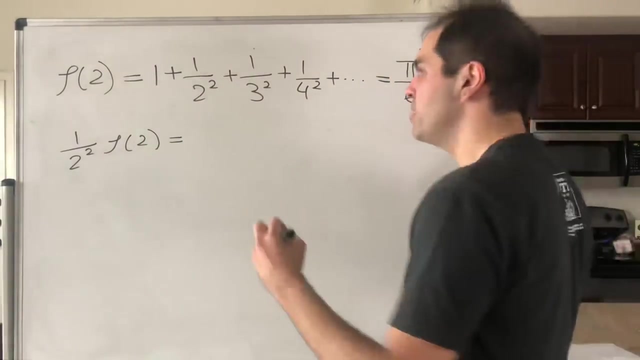 And let's apply the following clever calculation: What if we take zeta of 2 and we divide it by 2 squared? So let's do 1 over 2 squared zeta of 2.. Then it turns out what we get: all the denominators become even. 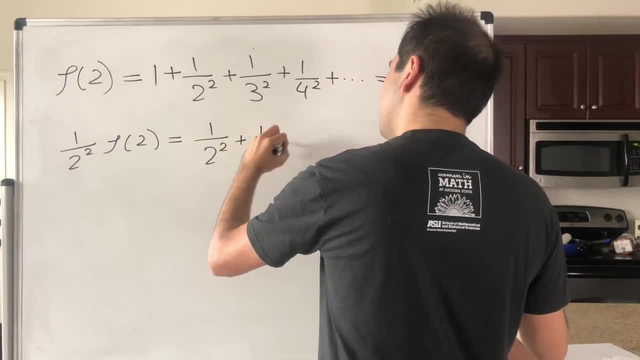 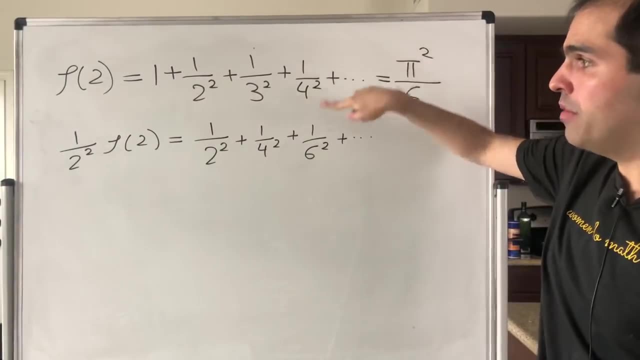 So it's 1 over 2 squared, plus 1 over 4 squared, plus 1 over 3 squared, 1 over 6 squared, plus dot, dot, dot. And now let's take the original sum and subtract it with this: 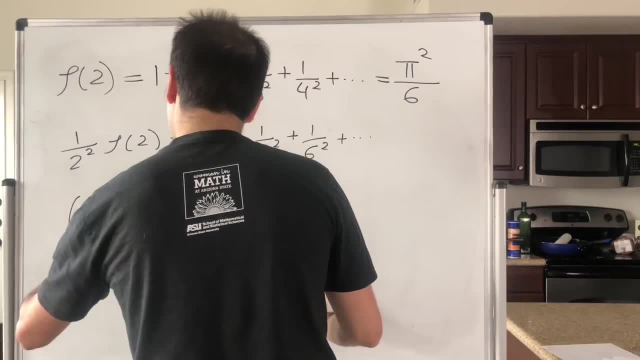 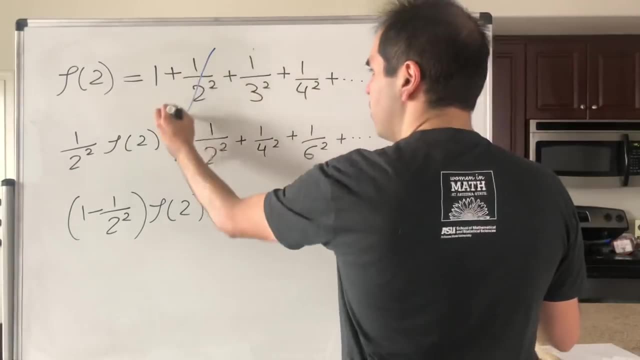 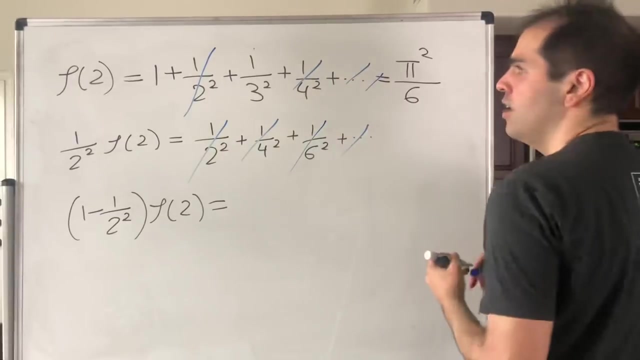 So let's try to do 1 minus 1 over 2 squared zeta of 2.. Then it turns out: if you subtract this from this, all the even terms disappear And what we're left with is simply 1 plus 1 over 2 squared zeta of 2.. 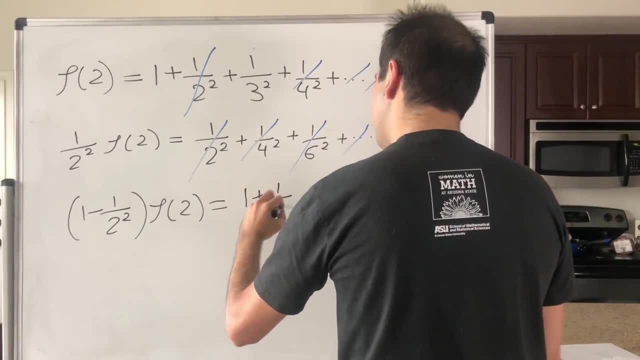 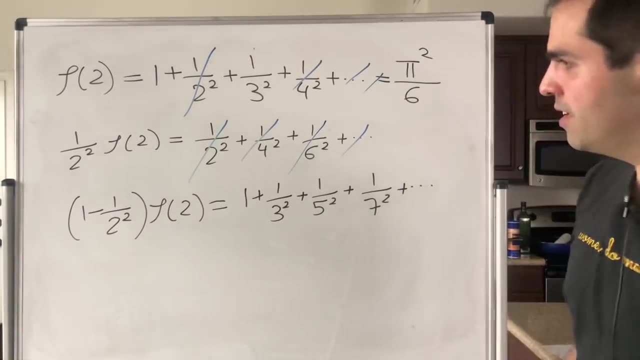 And what we're left with is simply 1 plus 1 over 2 squared, zeta of 2. Plus 1 over 3 squared, plus 1 over 5 squared, So all the odd terms, And it turns out if you do the same Spiel. 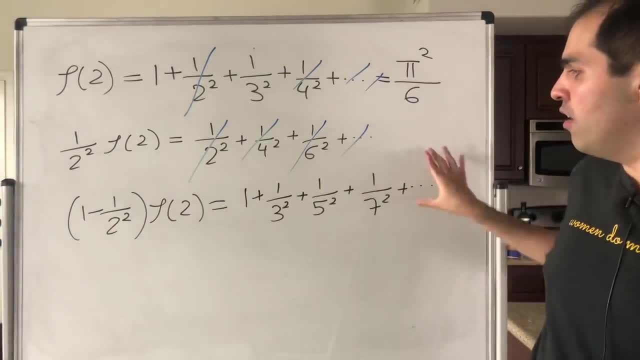 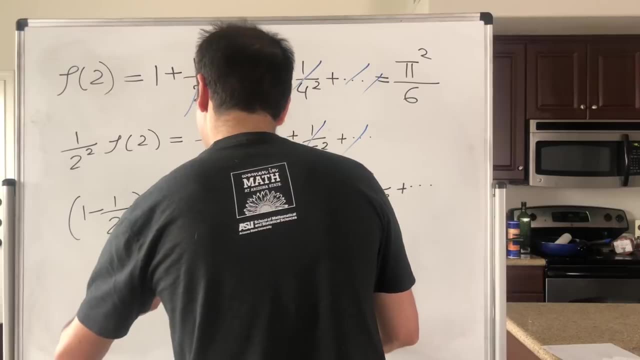 but with 1 minus 1 over 3 squared, then all the multiples of 3 will disappear. So in other words, zeta: 2 times 1 minus 1 over 2 squared, times 1 minus 1 over 3 squared. 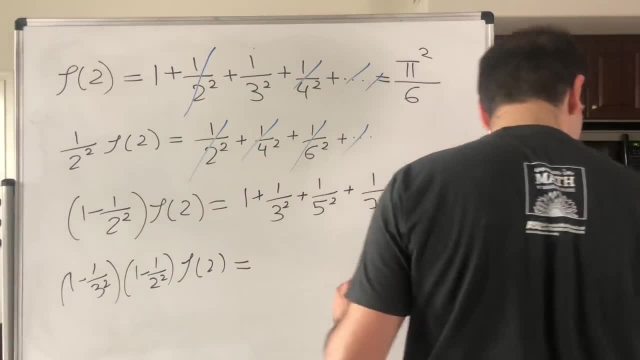 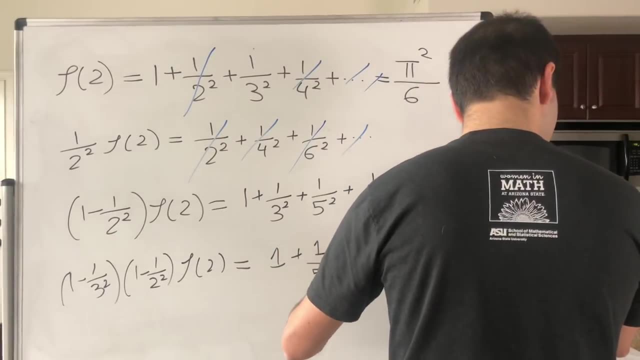 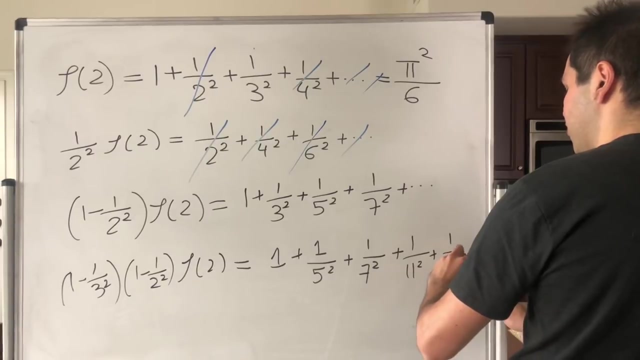 What this ends up being is simply, Let's say, 1 plus 1 over 5 squared, plus 1 over 7 squared, plus 1 over 11 squared, so not quite all the prime numbers, but you can have 1 over 35 squared, for instance, etc. 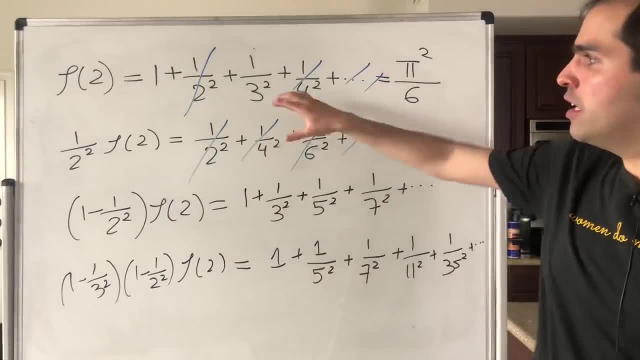 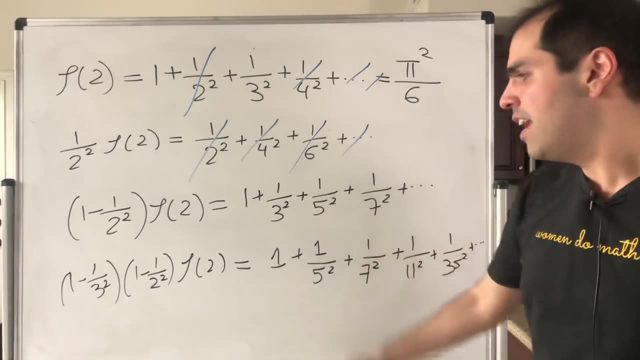 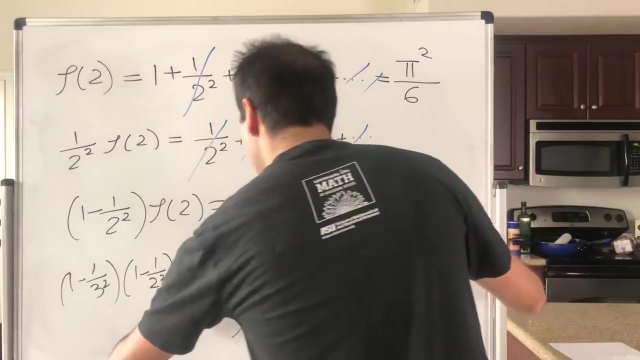 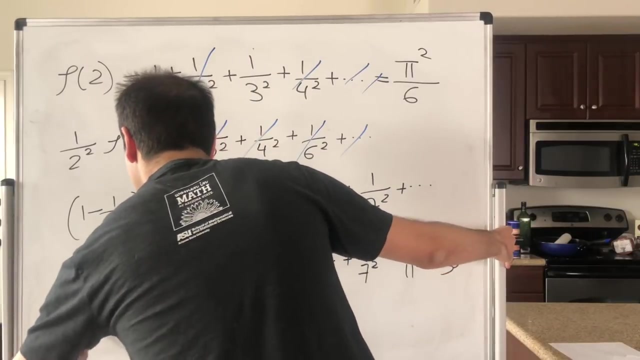 etc. and maybe now you notice the pattern. here we eliminated all the multiples of two, here we eliminated all the multiples of three. and it turns out, if you continue that process for every single prime number, so Zeta 2 times 1 minus 1 over 2 squared. times 1 minus 1 over 3 squared. times 1 minus 1 over 5 squared. 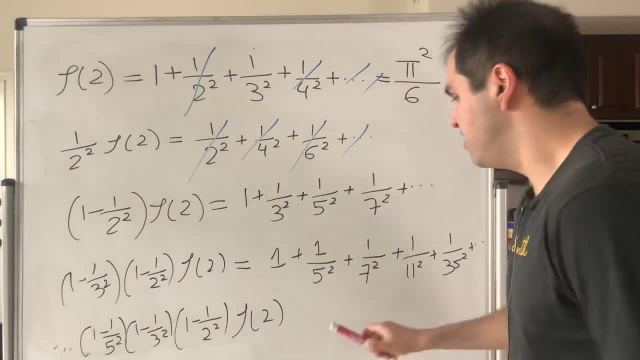 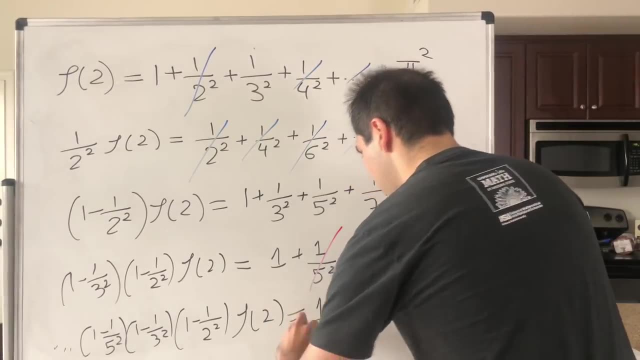 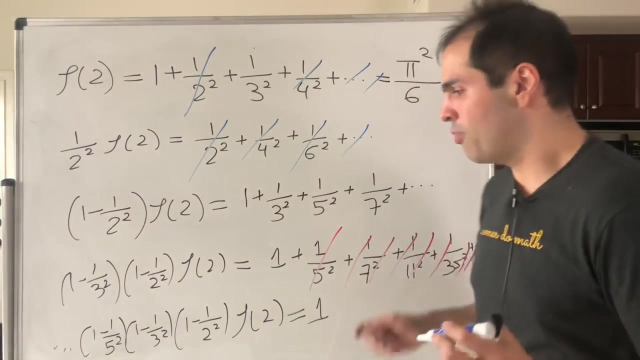 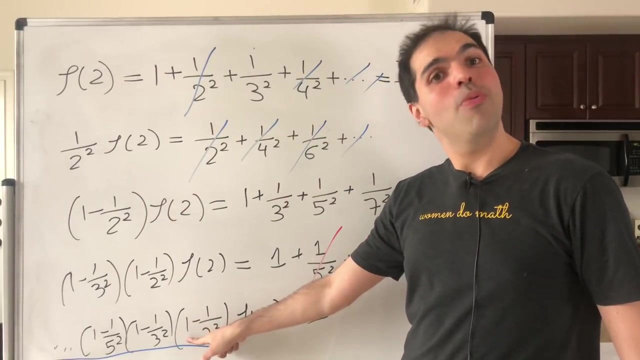 etc. etc. then everything disappears. so bang, bang, bang, bang, bang bang, except for this one. and you might say, okay, this is a random calculation. what does that have to do with the previous problem? this is precisely the probability that we wanted. so, in fact, now we actually have a closed-form. 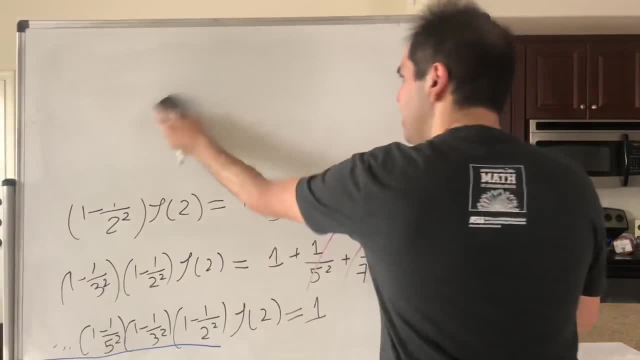 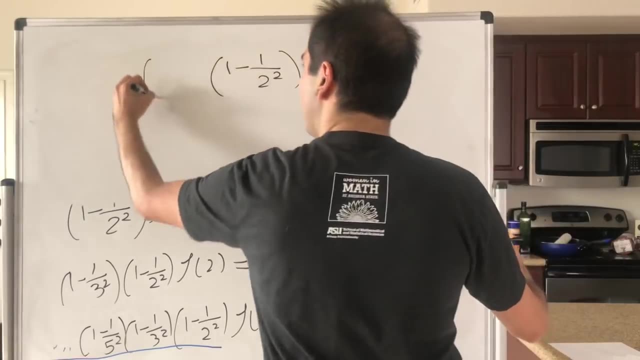 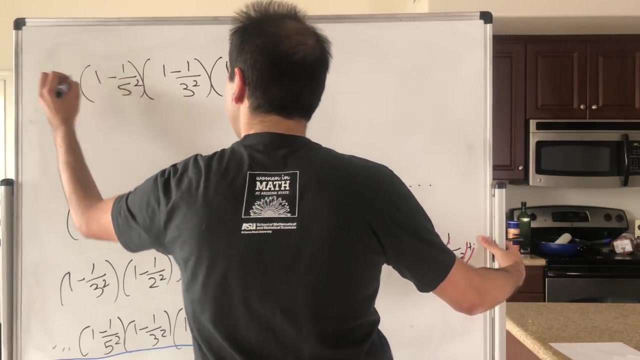 solution for our probability, namely again the chances of two integers being co-prime, which is 1 minus 1 over 2 squared, 1 minus 1 over 3 squared, 1 minus 1 over 5 squared, etc. etc. over all the prime numbers it's 1 over zeta 2, but remember zeta 2. 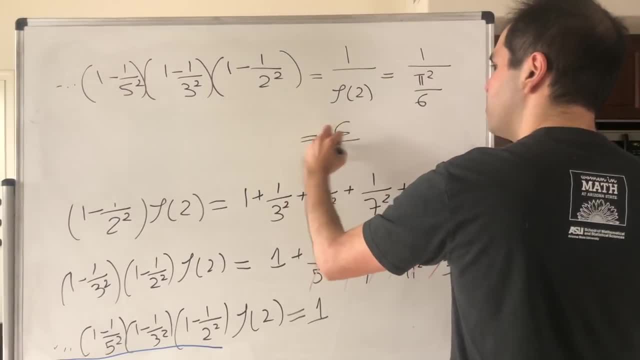 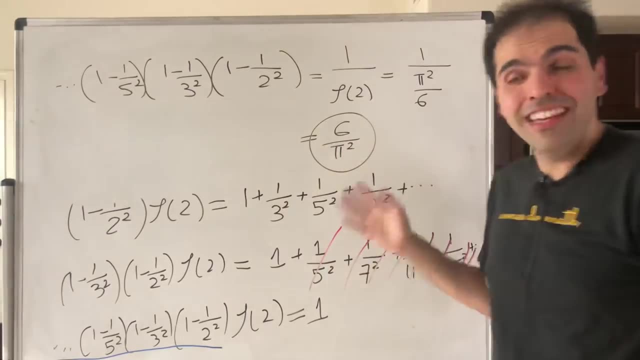 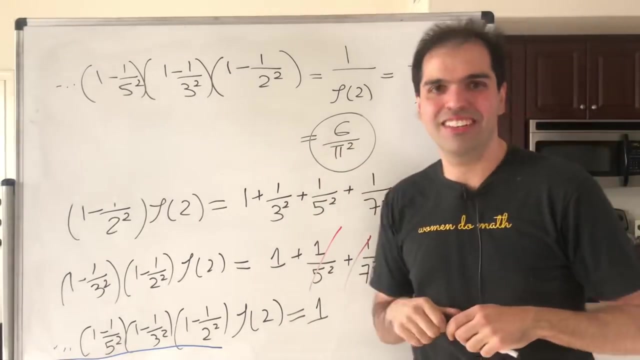 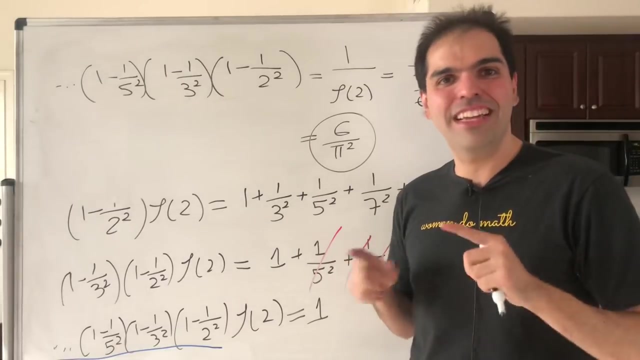 was pi squared over 6 and this is 6 over pi squared. did anyone guess that? probably not again. this is very, very neat. again, it's not obvious that co prime has to do with 6 over pi squared. but wait, we are not done, because it turns out there's an amazing geometric application of 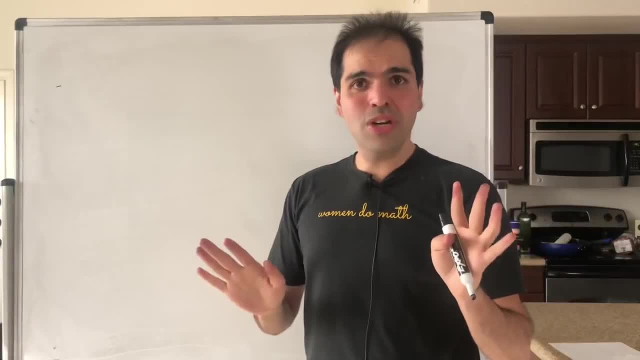 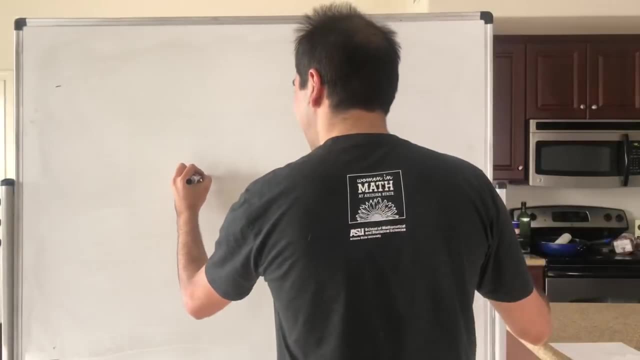 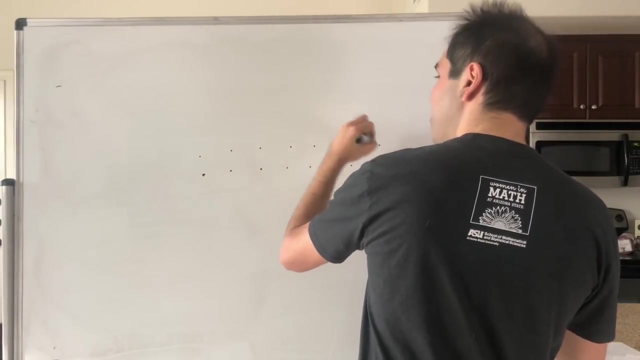 this, which i'll cover now. now let's try to cover another problem that seems to have nothing to do with co prime, namely consider the integer lattice, like that, so like this, so just the lattice of positive integers. and, by the way, so i got inspired by from this, by a tweet by juliet bruce. 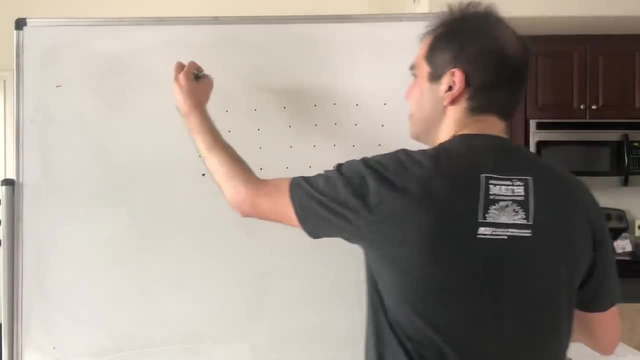 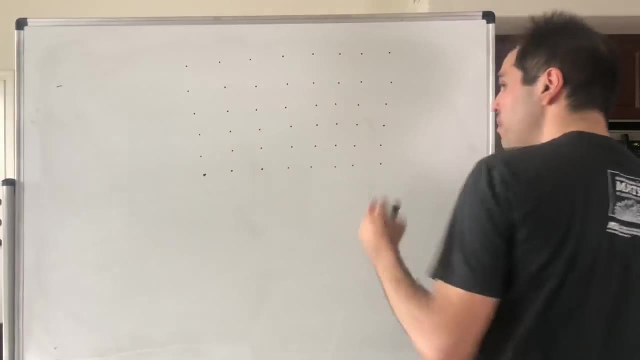 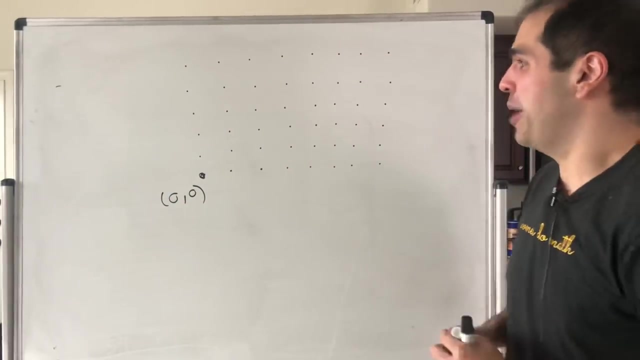 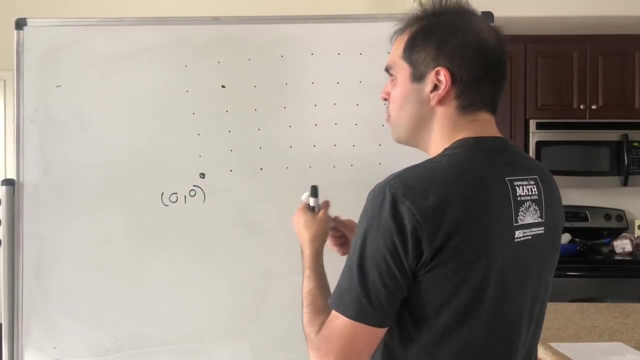 who talked about shadows and lattices and i was like, oh, i should probably do that. suppose you have the following lattice and let's say this is the origin: zero, zero. and let's consider the following fun game, namely, let's pick a random point and consider the ray going from the origin to that point. so, for instance, this is one, two, three. 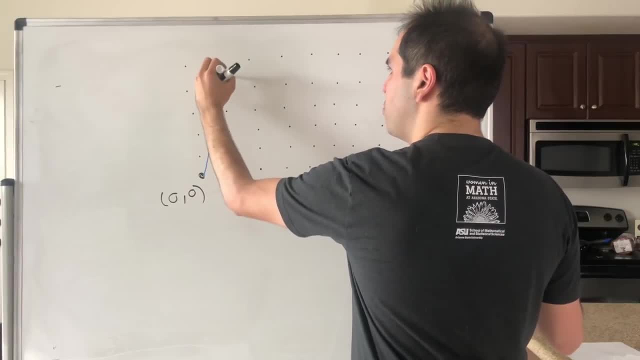 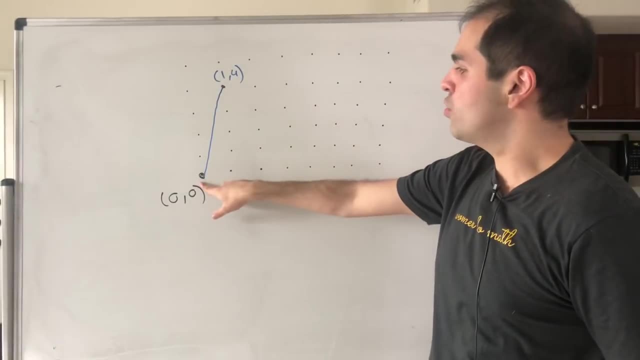 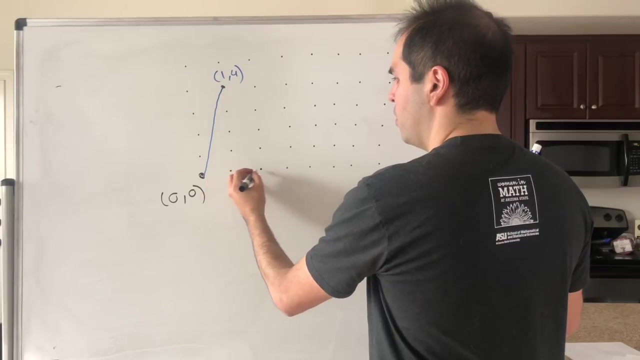 so one, two, three, four, so this is the point one comma four. but then, notice, here there's nothing blocking this ray, so this ray goes directly from this point to this point. but for instance, if we pick the point uh, let's say uh, zero, one, two. one, two, three, four, like let's say this point two comma four, then oh, 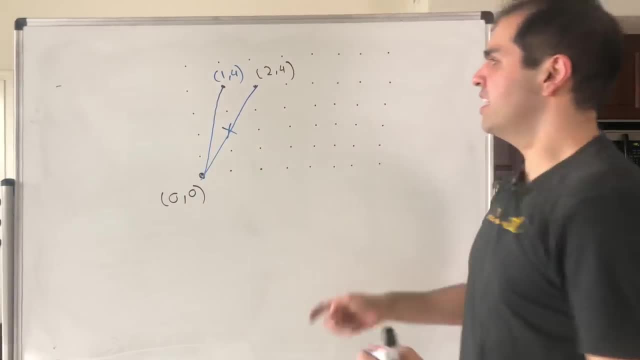 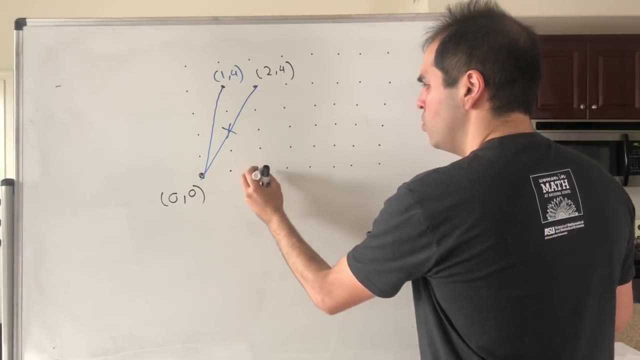 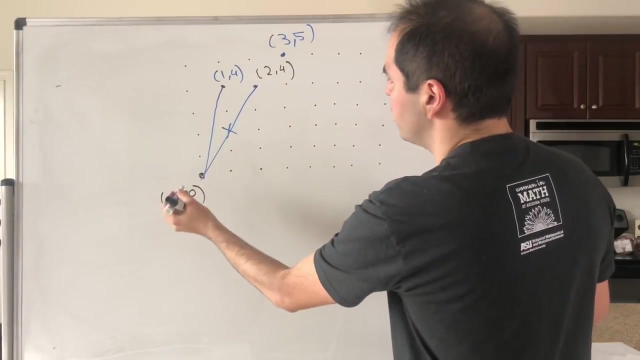 no, this middle point here is blocking the ray, so think like a kind of a shadow. but if we pick a, let's say the point one, two, three, one two, three, four, five, let's say here three comma five, then it turns out there's also nothing blocking that point. so kind of, if you have this ray, maybe it goes kind. 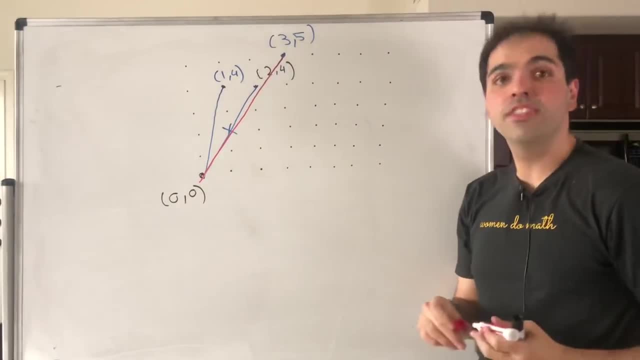 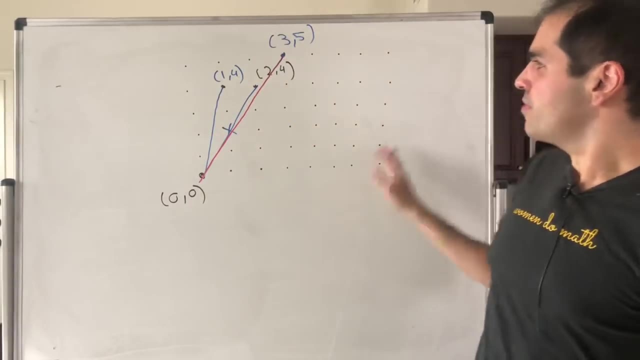 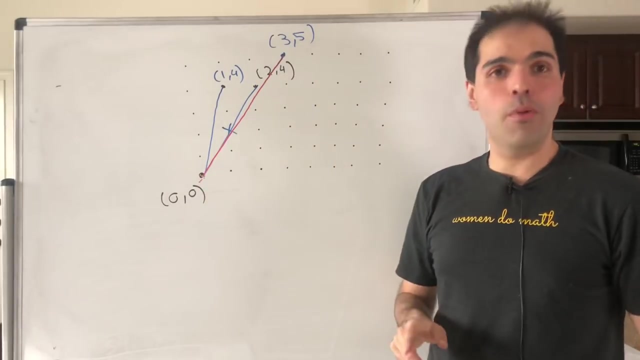 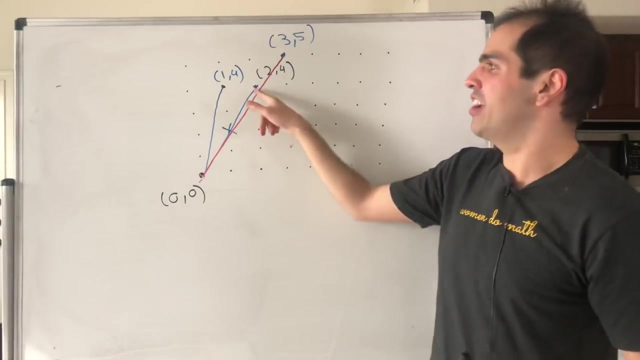 of like that, and notice it goes directly from zero, zero to uh three, five. and here's an interesting question, namely, um, what is the probability that, uh, a ray goes directly from a point to another? so, among any of those lattice points, what is the probability that there is no shadow there, or in other words, there is no blockage and it turns out? 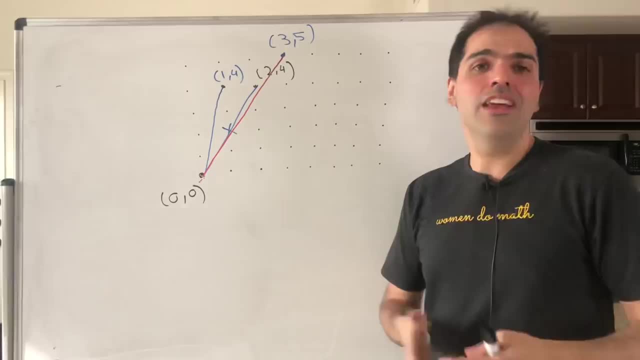 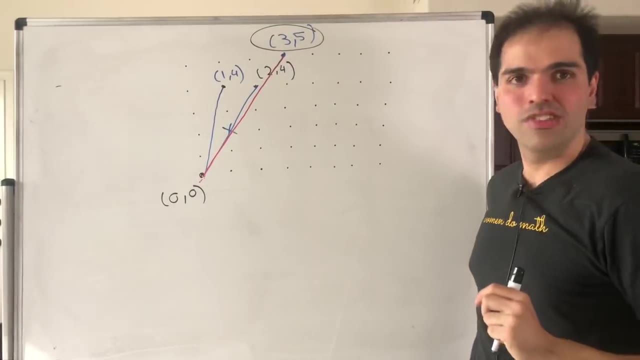 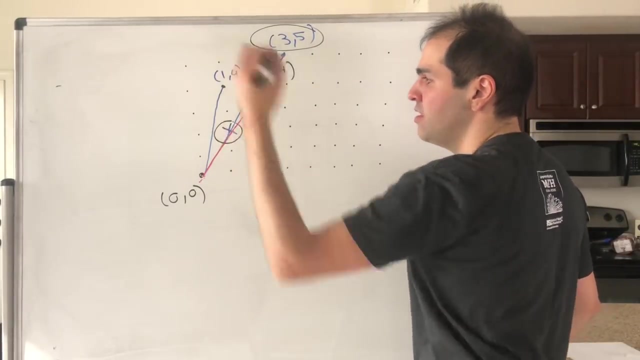 surprisingly it has to do with numbers being co-prime, because here, for instance, three, five, three and five have no factors in common, so there is no blocking. but if you pick, let's say, a, two, four, then precisely the point one comma two is blocking that ray, so in other words the probability.